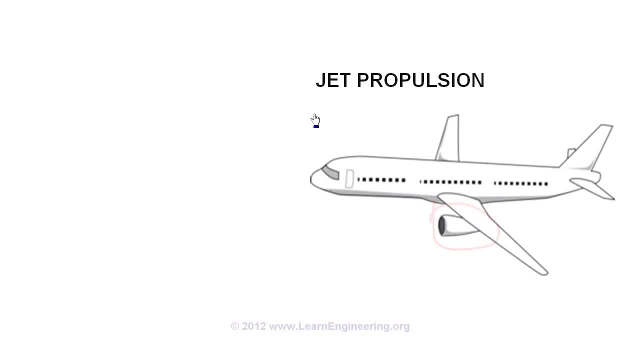 Let us understand how gas turbine engine is used for generating thrust force in an aircraft. Here is a close look of gas turbine engine of an aircraft. In order to make the flight move forward, this engine should produce a force in forward direction. This force is produced by jet effect of this exit fluid. 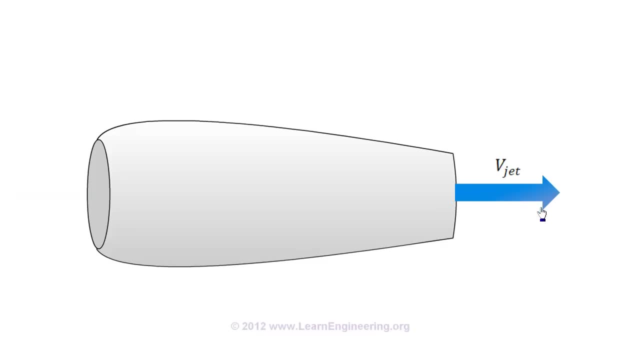 When a high velocity fluid is ejected the engine, it will produce a reaction force which will power the aircraft. This force is known as jet force. By applying Newton's second law of motion to jet engine control volume, one can easily find out magnitude of this jet force. 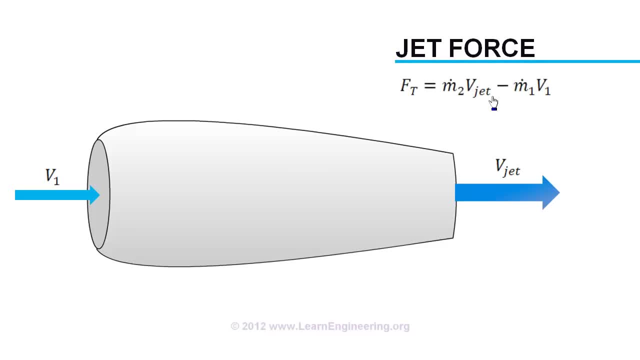 It is momentum at minus momentum in. So if jet velocity is high it means high jet force. This is why exit portion of a jet engine has got decreasing area if the flow is subsonic Or the exit portion acts like nozzle which increases jet velocity. 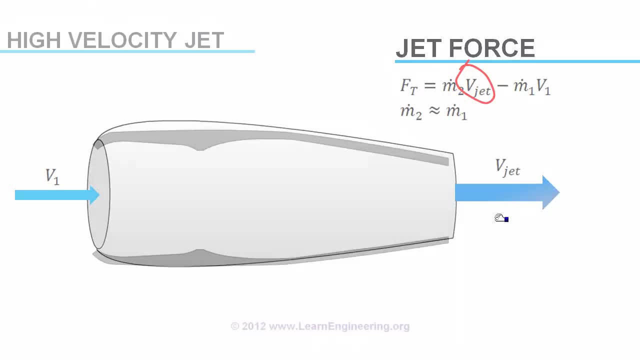 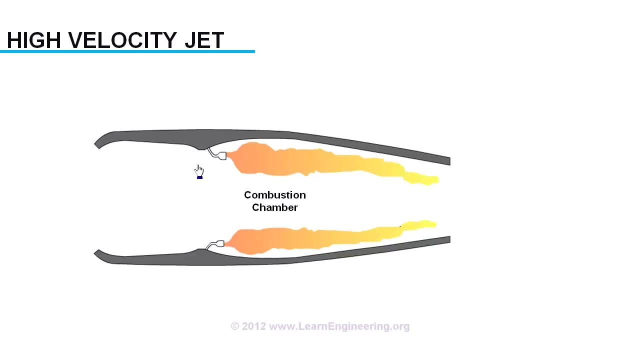 The million dollar question How to produce such a high velocity jet continuously. We will produce it by a combustion process, By injecting fuel into it Which will produce flames with very high velocity. But for a sustainable combustion process we need the inlet air to the combustion chamber to be at high temperature and pressure. 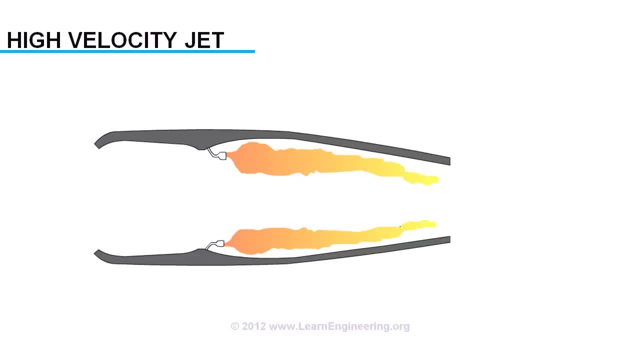 This is achieved with help of diffuser plus compressor arrangement. Air gets into the engine by forward motion of engine and sucking effect of compressor Diffuser increases pressure of this fluid to some extent by converting some part of kinetic energy to pressure energy. 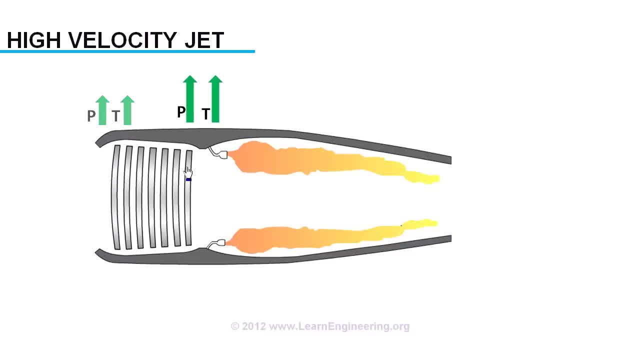 After that compressor comes where both pressure and temperature of the air is raised by energy addition from compressor. So at outlet of the compressor we will have air at high pressure and high temperature. But compressor requires some power input to do that. 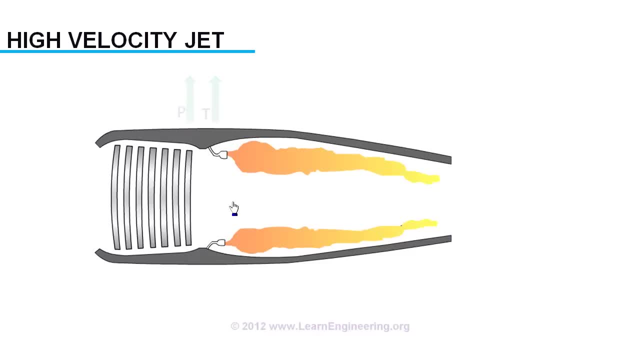 This power is given by a turbine which is situated right after the combustion chamber. The turbine absorbs some amount of energy from the high energy fluid and transmits it to the compressor. Thus the process of producing high velocity jet at outlet has become self sustainable.